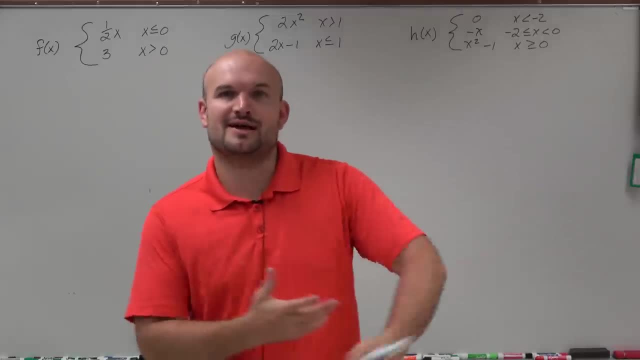 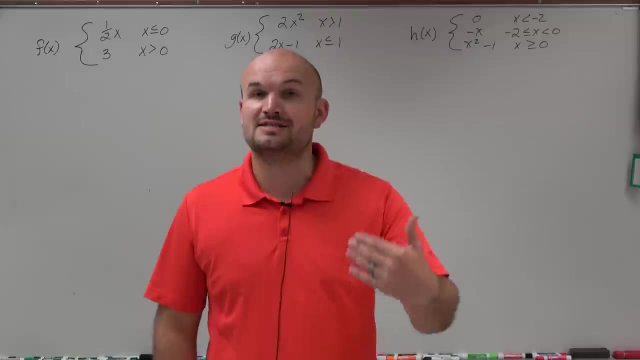 over here You have these inequalities, and it's not usually part of functions. It's like: what exactly does everything mean? So, basically, you know, to define a piecewise function, it's just a function comprised of two or more functions, So we don't really need to be, you know, so taken. 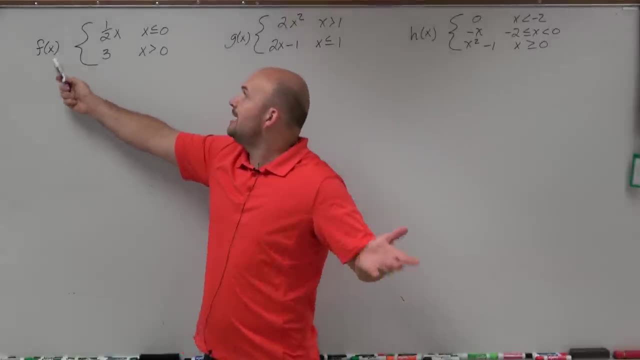 aback when we see a function f of x. right, That's the name of the function And you can see that it's comprised here of two different functions. So my first function is one- half of x, and my other function is three, where here I have two functions and then here I have three functions. 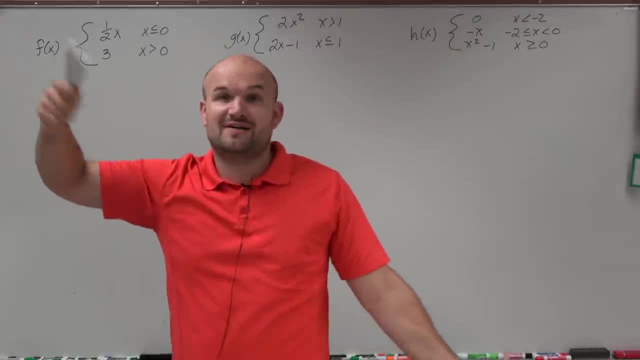 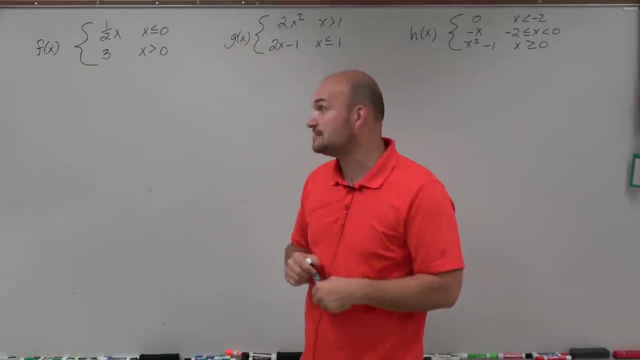 So you could even do piecewise functions that are, you know, made up of four or five, six. but we're going to kind of keep this kind of simple video and just deal with a couple functions. Now, when graphing functions, basically all we're simply doing is graphing each of. 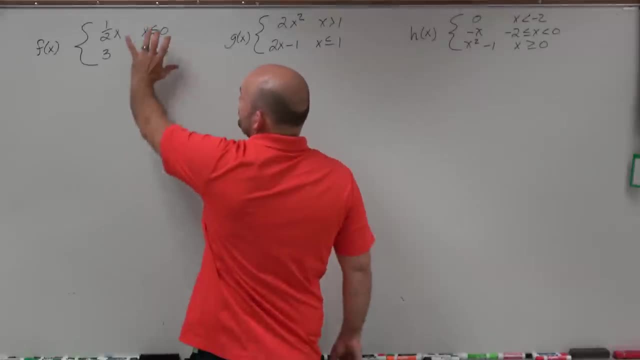 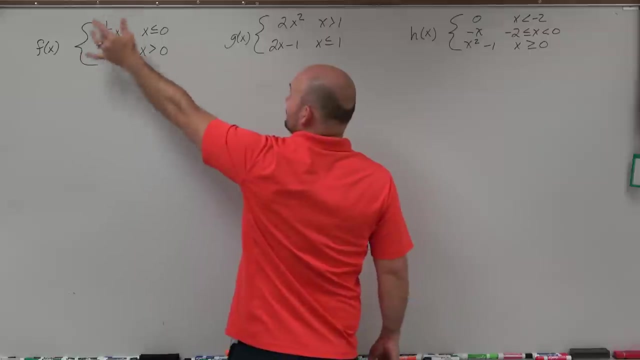 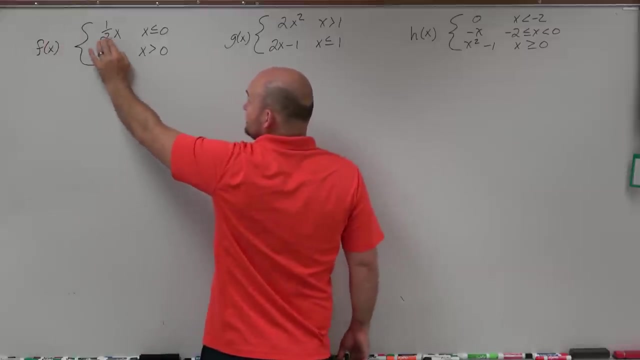 those functions correctly and then abiding by the constraint. So what the function? what this piecewise function means is this: f of x function. the value of the f of x function is one half x for only input values Because, remember, like here's our function, f of x, that's our input. So we're 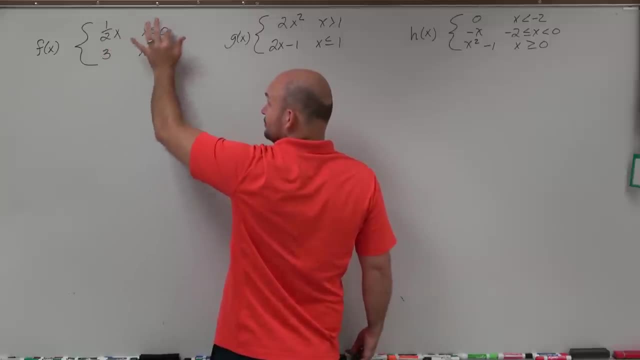 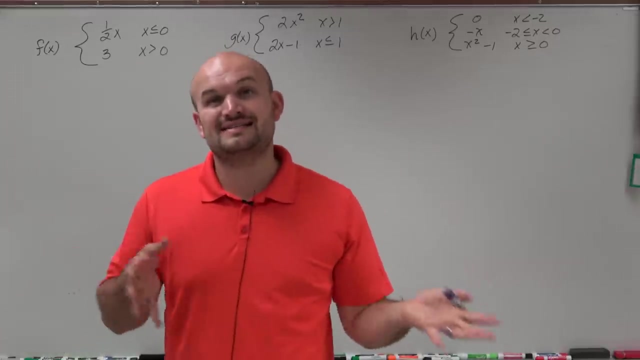 only going to use this function for input values, or x values that are less than or equal to zero, And we're going to use the bottom function for only values that are greater than zero. So to do this, I'm going to use a few different ways I like to do it. The first way is just to graph each 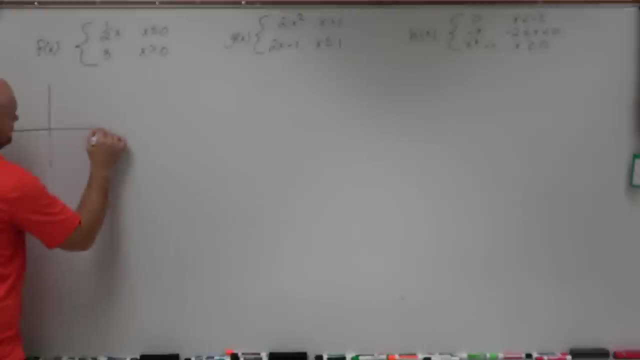 function that you have separately. And this is just kind of like an introductory way. It takes usually a little bit longer to do, but I think it's like a really important way just to understand what exactly are we graphing. And you got to obviously know how to graph. you know functions. 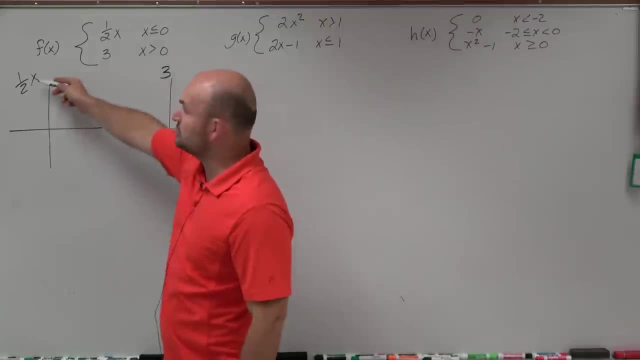 to be able to graph the piecewise function. So the first function is one half x, And forget about the constraint. I think the constraints usually confuse a lot of people, So let's just forget about the constraint and say: all right, what is one half x? 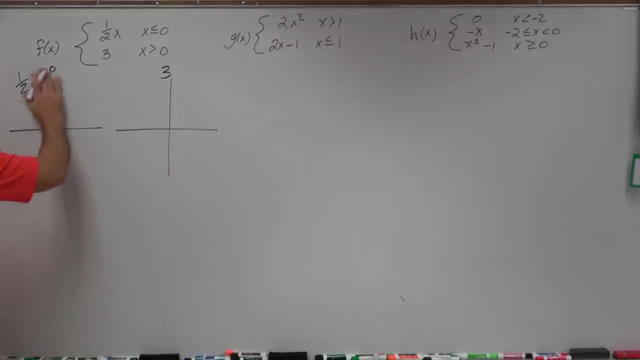 Well, remember, that's basically a line. So you could say one half x. I'll put this: you know, plus zero, y equals mx plus b, right? So we have a y intercept at zero, And then we're going to rise, one over two, up one over two, or you could go down one to the left, two right. 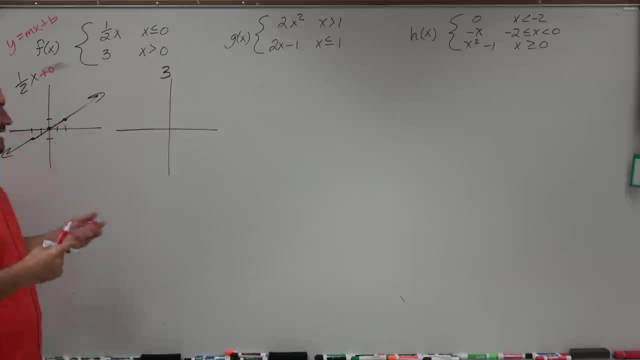 And let's just do a couple points just to kind of get a line, And that's perfect. That's all we need. For the next one is: we have a function at three And when you have just a value at three, basically that's going to be your y value, your output value is at three One. 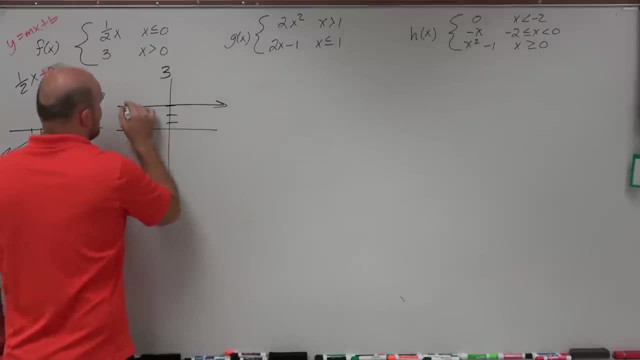 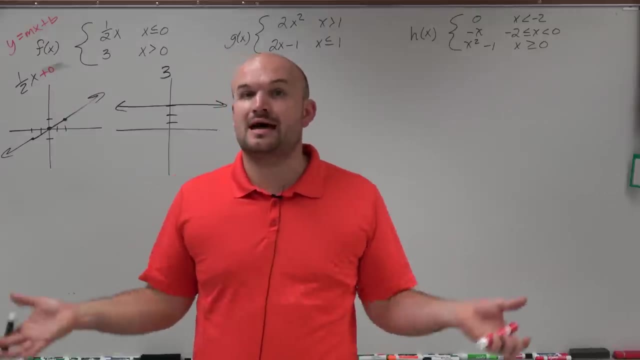 two, three, And you're just going to have a nice little horizontal line. Okay, So that's what these two functions look like separately. Now, all we're simply going to do is bring them together. However, before we bring them together, what's important is for us to be able to kind of 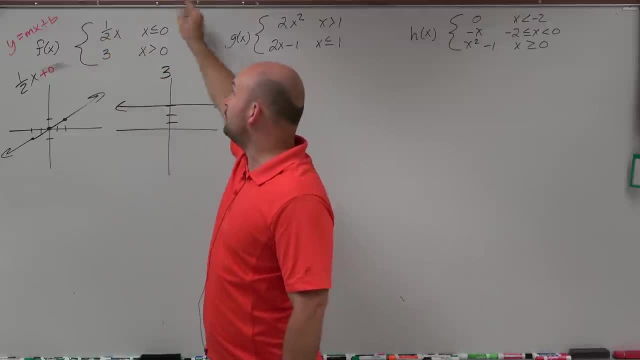 look at these and say, all right, I'm graphing the one half x, but I'm only graphing when x is less than zero. So if you think about a number line like: here's positive, two, here's negative, two right, Here's. 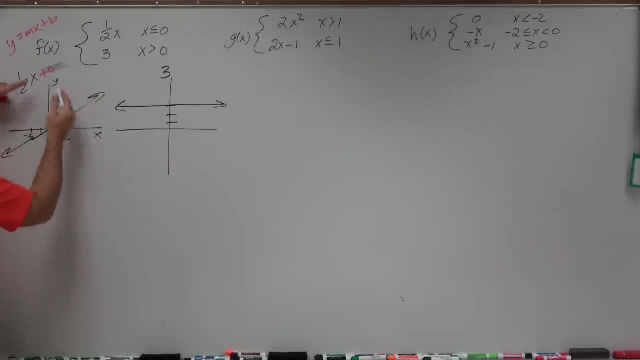 the x-axis. here's the y-axis. So when x's are less than zero, that's going to be from the y-axis over. So, in reality, all we need to do is we're not going to draw anything that's positive. 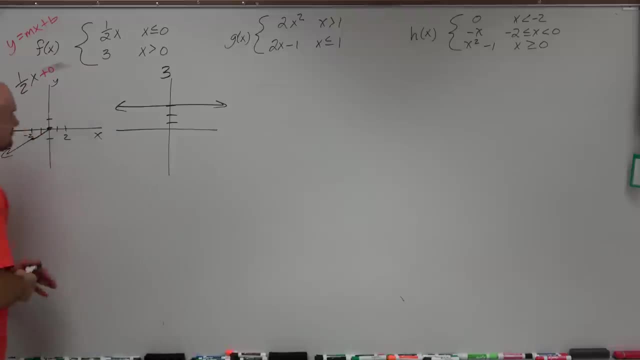 where the x values are positive, only when the x values are negative And that's greater than or equal to. so that is going to be filled in. Here we're only graphing three, the function three, for x values that are greater than zero. 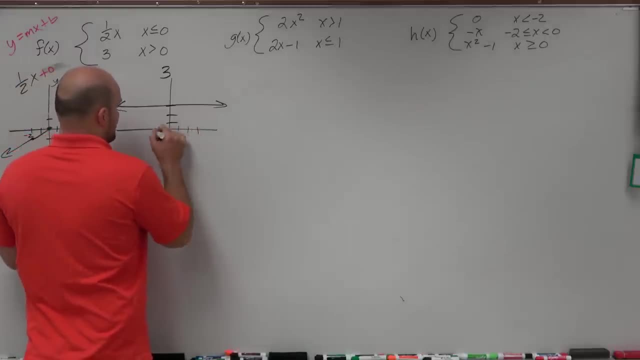 Well, again, here's 1, 2, 3, 1, 2, 3, negative 1, negative 2, negative 3, 1, 2, 3.. We're only graphing for values that are greater than zero, So that's going to be for all the positive. 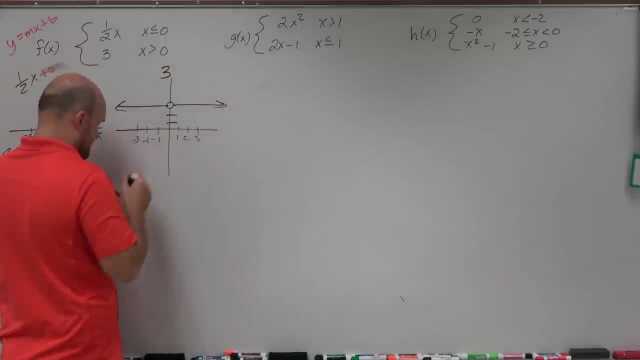 values, But it's not greater than or equal to, so zero is not included. So we're going to use an open circle And then we're going to go ahead and delete them. Now, basically, what we do now that we've grabbed them separately and added in their constraint, we just combine. 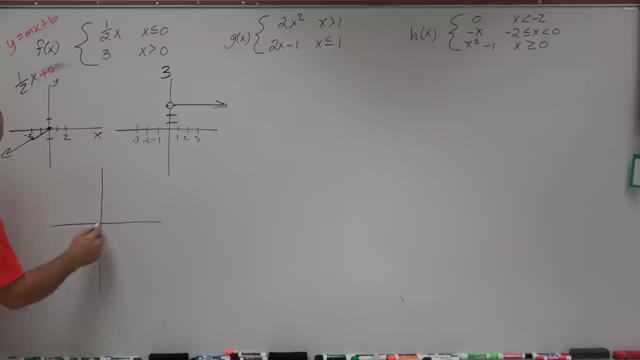 them into one graph. So I'd say, all right down here, down 1, over, 2, graph, And then 1,, 2,, 3,, open circle, Boom, And there you go. All right, So the next one is now. we have a quadratic here And we have another linear. 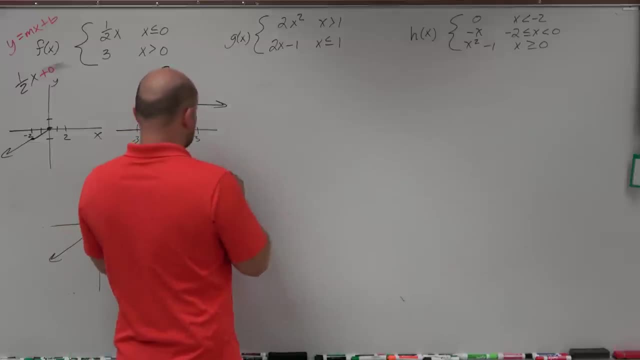 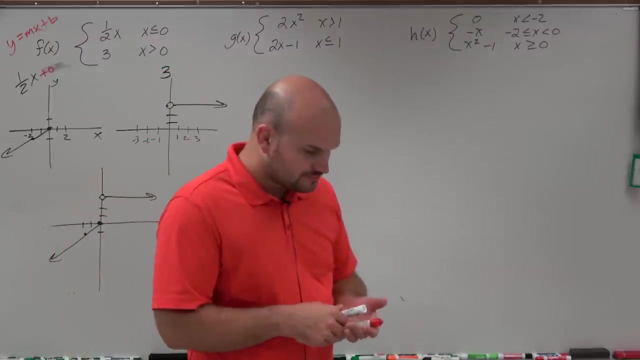 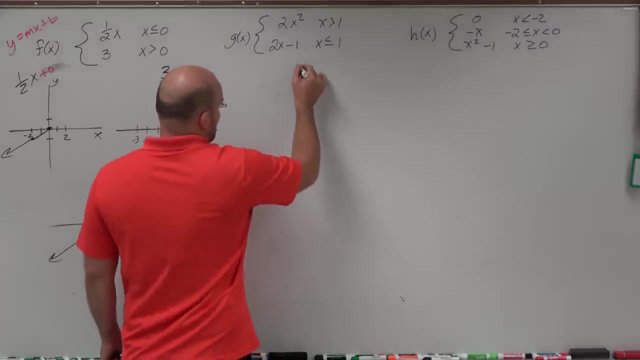 equation y equals mx plus b, Or mx plus b, I guess you could think about that. So again, as far as quadratics, You know, it's really helpful just to kind of know what the parent function is. The other way we can do this is just by graphing them together on the same. You could use different. 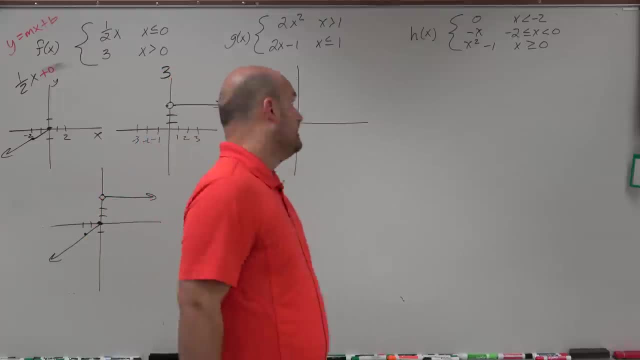 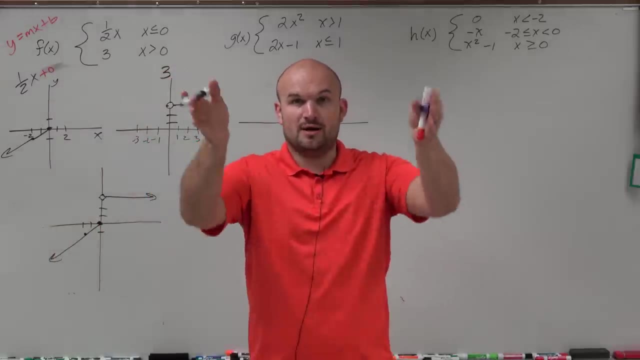 marker colors, but I really don't see a problem with just using kind of the same. So let's go and do 2x squared. Now we know that x squared is going, you know, starts at 0,, 0, and then goes over 1,. 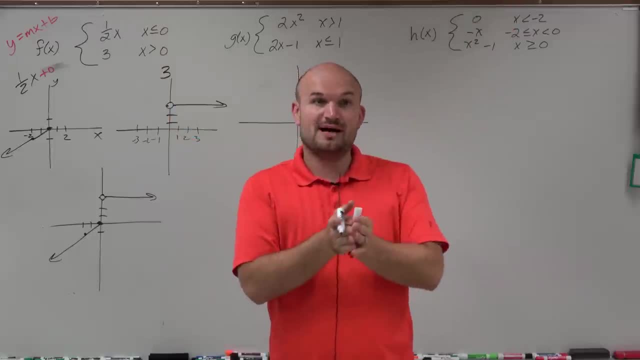 up 1, and then over 2,, you know, up 4.. So if you're multiplying that by 2, that's basically stretching that as a power of 2.. So it's going to go over 1,, up 2, and to the left, 1.. And 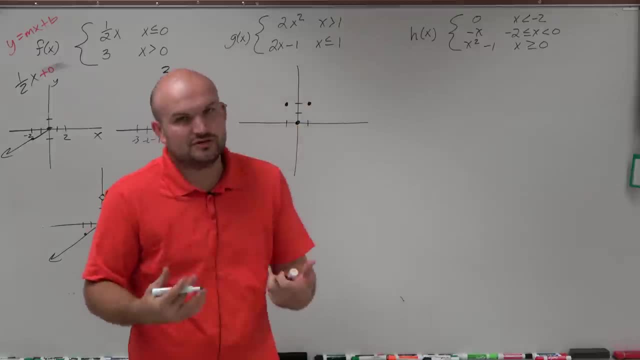 to the left, 1, up, 2.. And again the really purpose of this. I mean you should know how to graph a lot of these, you know by hand. I mean, I chose some very simple functions, So make sure that you have at least the basics of graphing. However, this could also be that 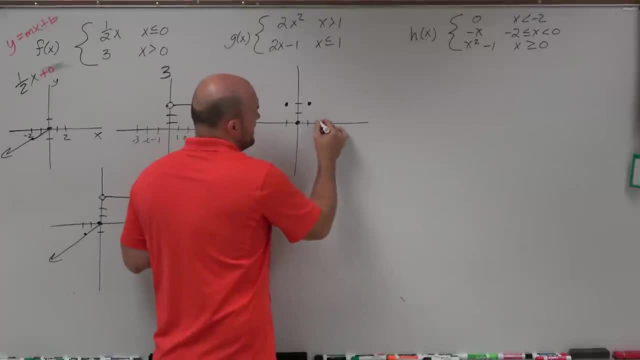 you know, if you're a lot of technology, you know you could verify my results as well. So therefore, it's going to be over 2, up 4, but then times 2. So it would be over 2,. 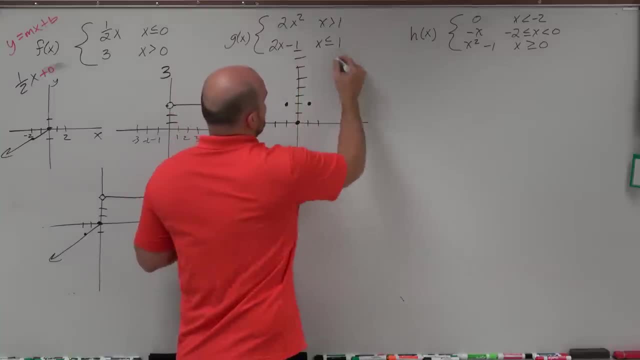 up 8.. 1,, 2,, 3,, 4,, 5,, 6,, 7,, 8.. So it's going to be like really really high up there, And you can see this is basically stretched. 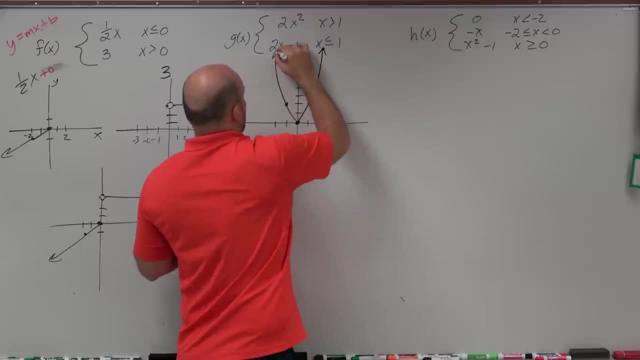 Boom right, And I think it's also important when doing this method, or even on that method, is to you know, make sure you use an eraser. All right, the next one is 2x minus 1. So 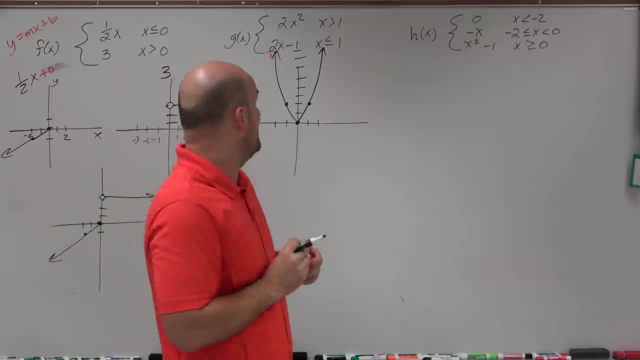 just remember, think of 2 over 1 as your slope And then minus 1 would be your y-intercept. So we go to the y-intercept and then we go up 2 over 1, up 2 over 1.. You could also go. 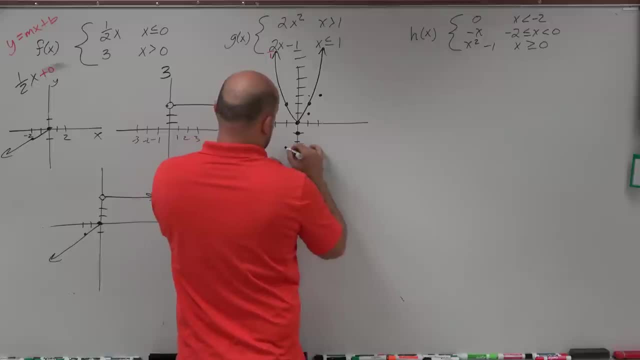 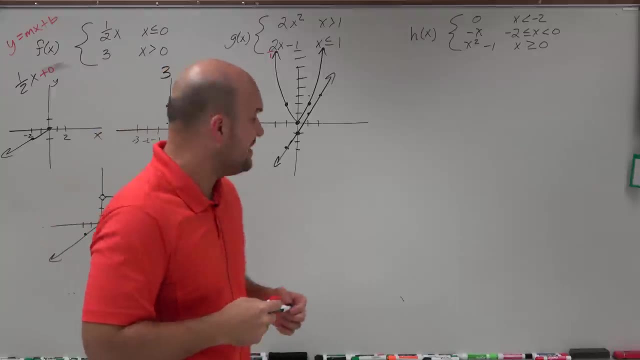 to the left Down, 2 over 1.. OK, So that's what our two graphs separately look like, And then we basically just kind of go where our constraint is. So we're only going to be 2x squared when x is greater than 1.. 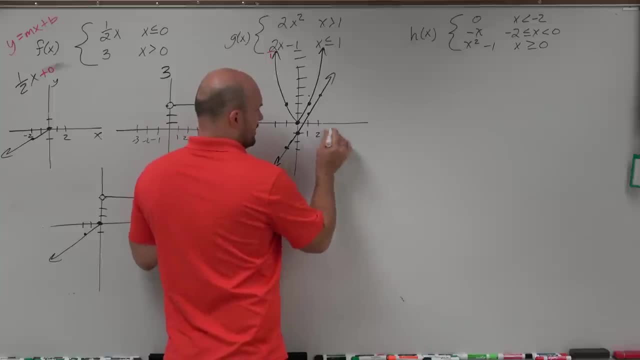 So we go to where 1 is and you could say: here's 1. Right, Greater than 1 is going to the right, Less than 1 is going to the left. So this is saying you're only going to use. 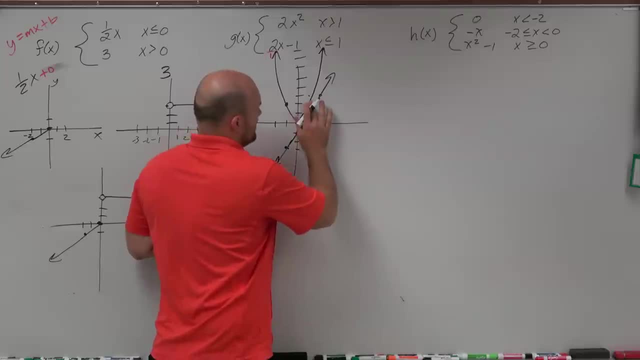 2x squared when x is greater than 1.. So first of all, it's greater than, not greater than equal to. We're going to use an open circle and we're going to go to the right. That means all the. 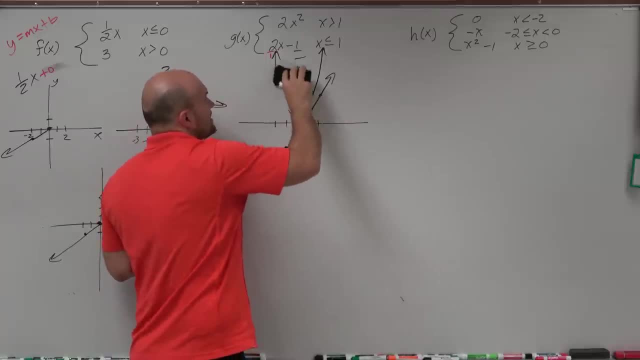 rest of this graph that I just did is not a part of the piecewise function. Yes, it's a part of the function 2x squared, but that is being constrained by when, for only values that are x is greater than 1.. Here is x is less than or equal to 1.. So it's going to 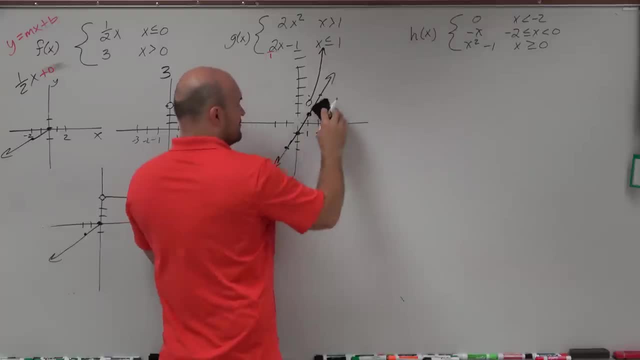 be a closed circle here and then it's going to be everything going that's less than 1.. So the rest of this we're just going to erase. OK, And just make sure, guys, based on the inequality symbol, you'll know if it's going. 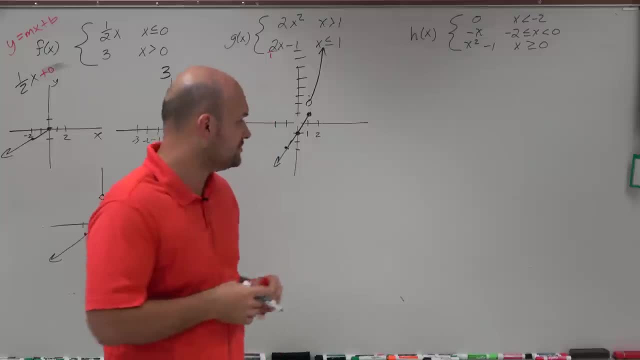 to be equal to or mean open or a closed circle, All right. and then, last but not least, here we have h of x, which is comprised of three different functions, And again, the same exact thing. What I'm going to want to do here is: 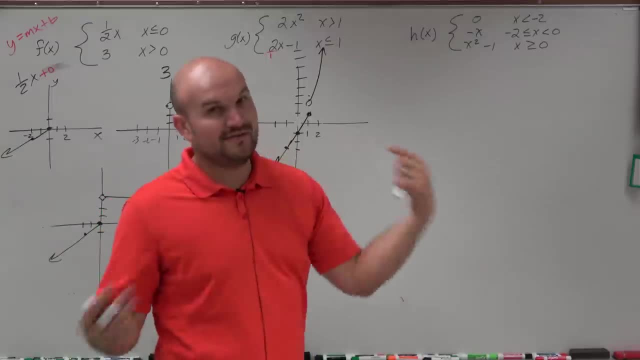 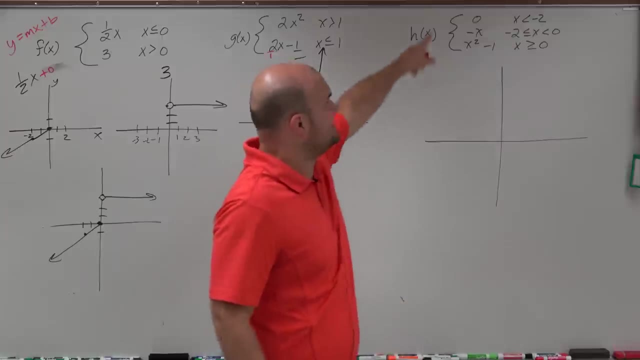 just graph each one of these separate, or graph them separately on the same graph and then kind of erase based on their constraints. All right, the first kind of constraint is kind of hard to see because it's 0. Well, if here's y, here's x, the output is 0. That. 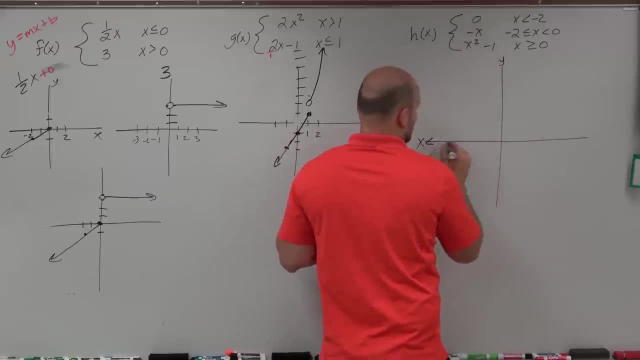 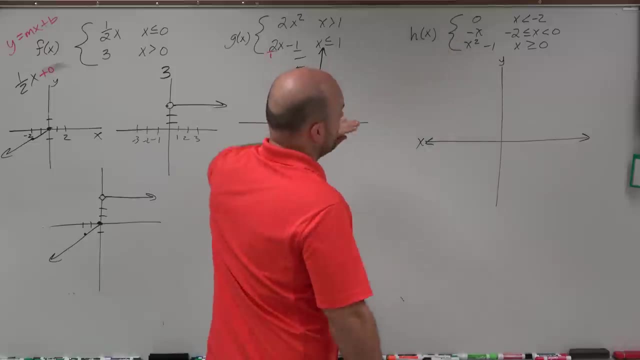 means it's on the x-axis. So that's kind of a little bit hard to understand or see because it is on the axis, but we'll say that is where it's at. The next one is negative x. So we know that positive x is that identity function So negative. 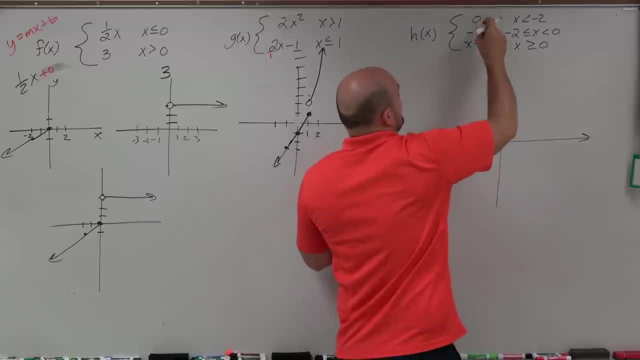 x is going to be the identity function. You could think of the slope as 1 over 1.. So you could go over 1, down 1.. Or you could go up 1 to the left, 1.. But just remember that it's. 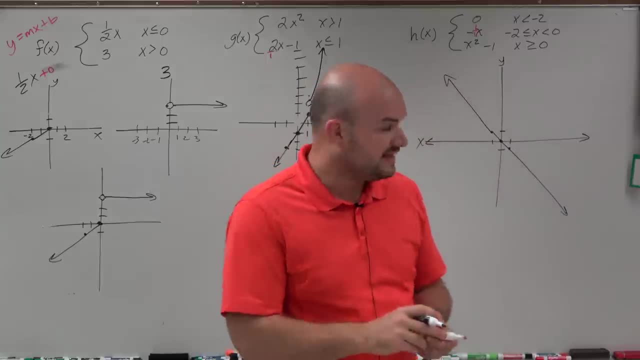 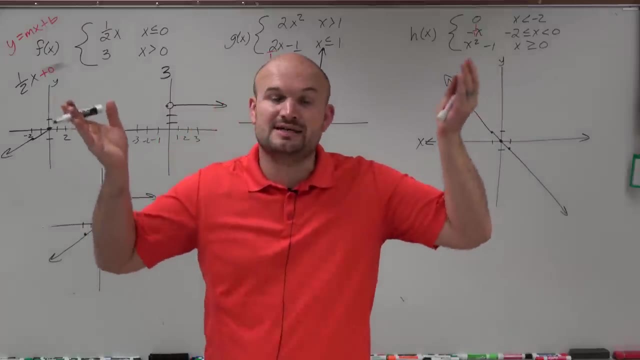 going to be going down and to the right, And then, last but not least, we have an x squared minus 1.. All right, so that's going to be another parabola, And the only thing different now is there's no stretching. 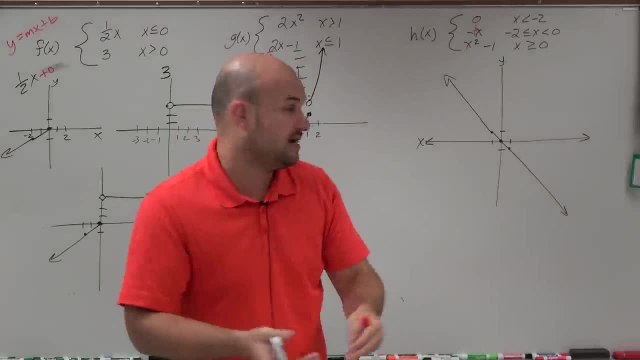 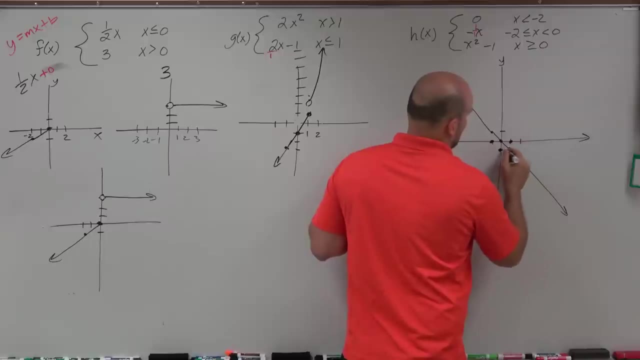 So it's over 1, up 1, over 2, up 4.. But now it's being shifted down 1.. So you can see, here there's going to be your vertex Boom over 1.. Let's go over 2, up 4.. 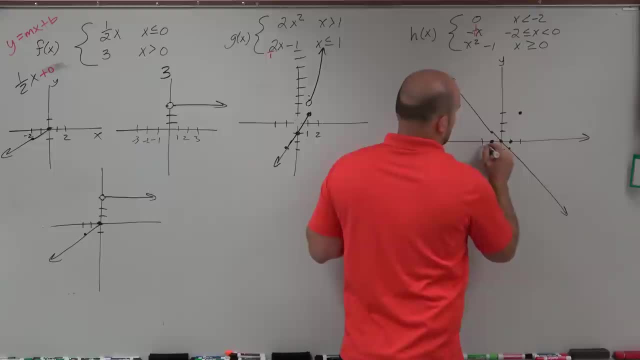 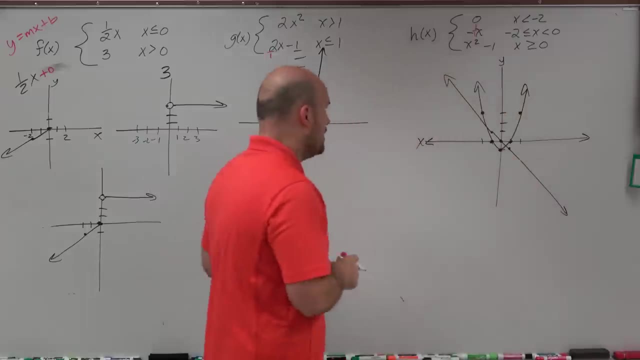 1,, 2,, 3,, 4.. Over 2,, up 4.. OK, All right, so we have three functions. We have 0, negative x and x squared minus 1.. Now what we simply need to do is go ahead. 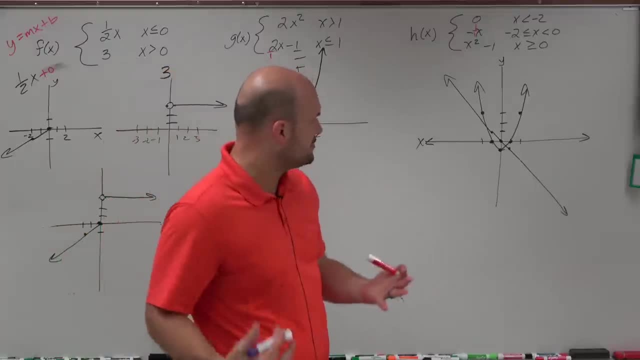 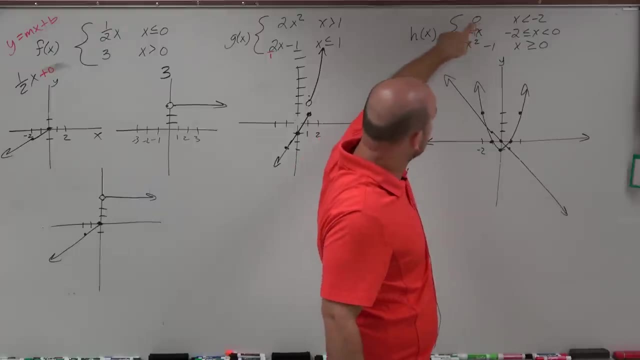 and go back to our constraints and then now eliminate each function based on the constraint. So here's negative 2, and that's going to be basically where all my constraints are changing. So this one says: you're going to use 0 for x. 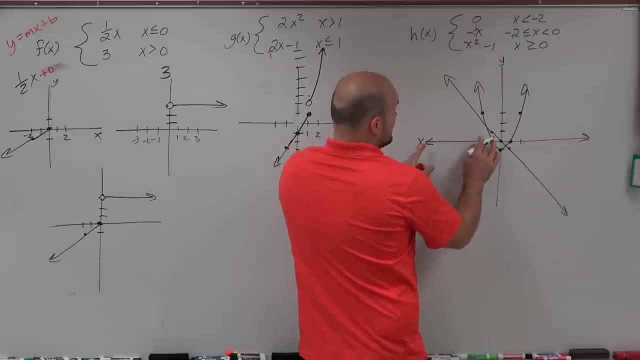 is less than negative 2.. So it's going to be this function, It's going to be an open circle, and that's for all values that are less than negative 2.. Then we go to the next one: negative x. That is true for all values that negative x is right here. 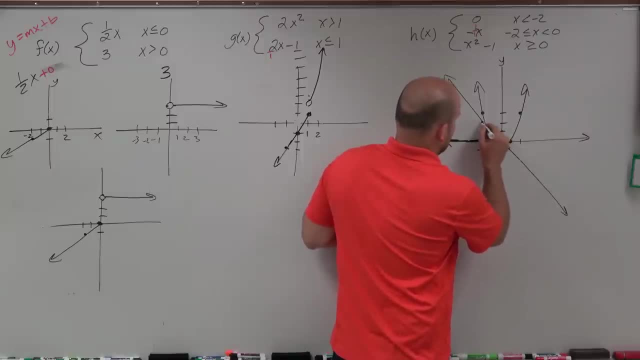 So that's over 1, up 1, and then let's see: over 1, up 1.. So there's another point right there. So it's going to be from negative 2 to x equals 0. So again, x equals 0 at the origin. 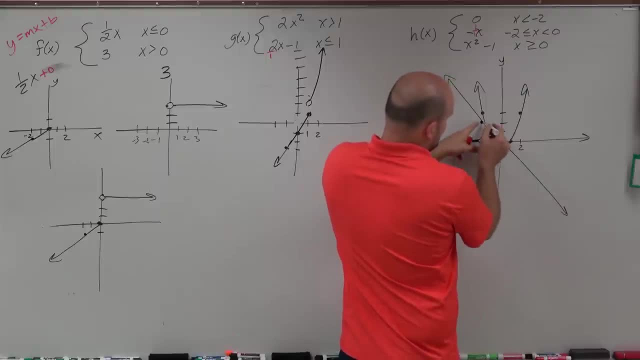 and x equals positive 2 over here. So you could do negative 2 to 0. So it's only between these two values. Here is a closed dot, but at 0 it's going to be a open dot. So everything else. 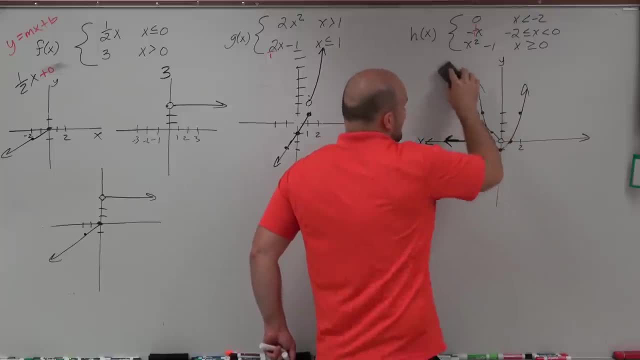 Is going to need to be erased, Only values between negative 2 and 0.. And again, it's the x values, right? A lot of people get confused with the y values, Not the y values. It's when x is between negative 2 and 0.. 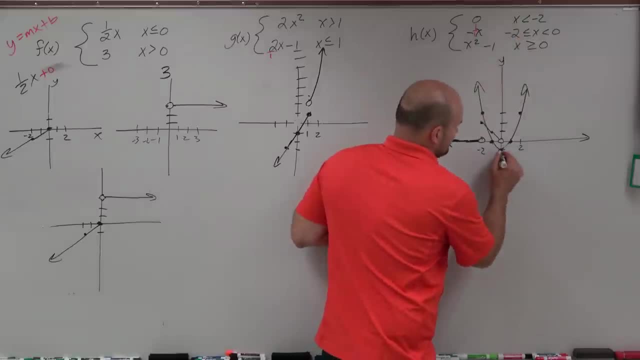 And then here it's, for x is greater than or equal to 0. So here's, x is at 0, and that's going to be everything going positive. So we're just going to erase everything over here, And there you go. 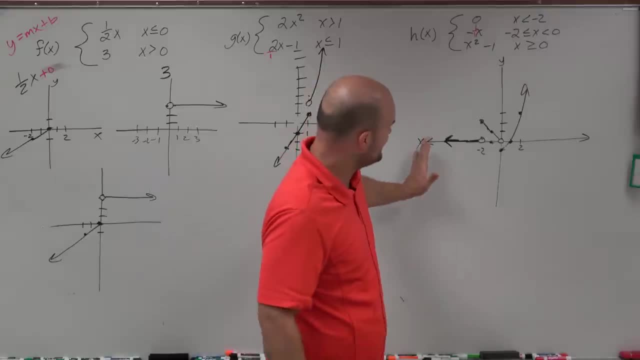 And again notice that, on each one of these values, this still passes the vertical line test, Because, even though we have two points here, this is contained, This is not contained. This is not contained, This is contained, So it still passes the vertical line test.